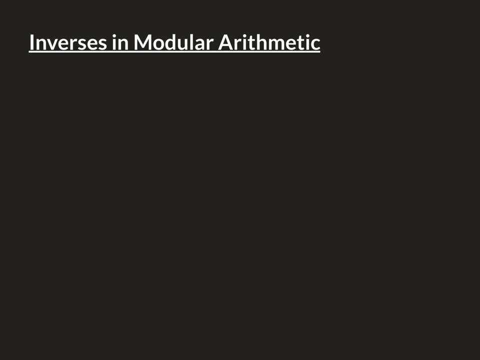 So in this video we are going to use Bazut's identity, which is a result in number theory, to understand which elements inside the ring of integers modulo n have multiplicative inverses. So Bazut's identity is absolutely crucial prerequisite knowledge to be able to watch. 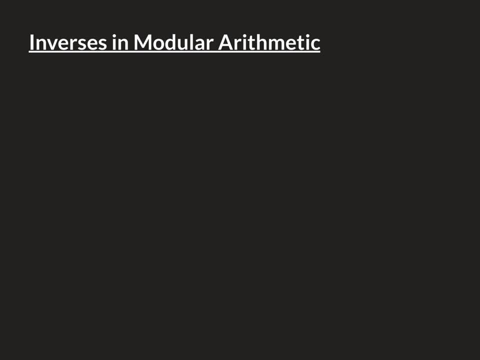 and understand what we do in this video. So if you aren't familiar with that result, please go to my playlist on number theory And in that playlist there is a video on Bazut's identity. Please watch that video before returning to this video. We proved: 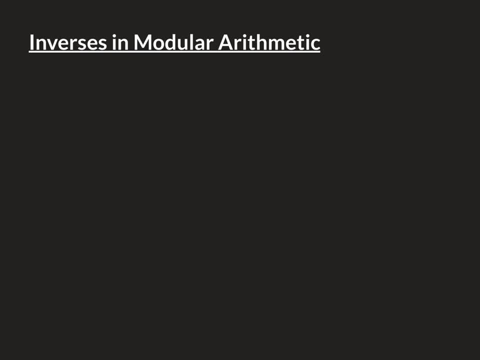 the Bazut's identity in that video. So, going forth, I will assume that everyone is familiar with that result. So we're going to be talking about the ring of integers modulo n, which I will denote Zn, And we're not going to pick a specific n. What we're going to say is going: 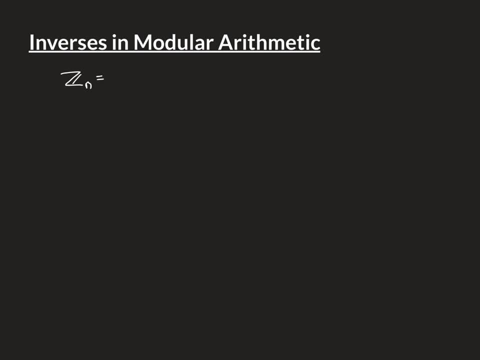 to apply for all of them. So remember this, as a set is a finite set and it will contain the elements 0,, 1,, 2,, all the way up to n minus 1.. And this set will have two composition laws defined on it: an addition composition law and a multiplication. 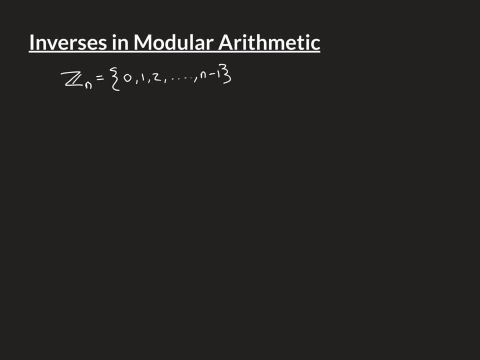 composition law And remember the way those composition laws are defined, is you think about each of these elements as representing a congruence, class modulo n, in the larger ring of integers? And then, if you want to know what any two elements added together, or any two elements, 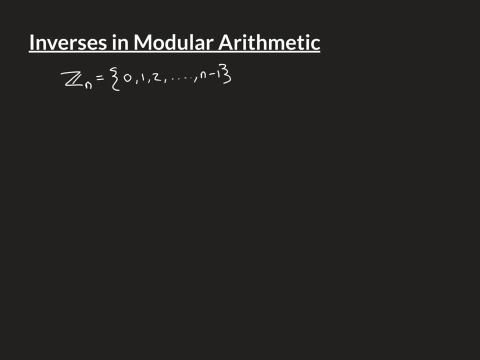 multiplied together? is you think about going to their congruence classes, picking representatives out of them, adding those representatives together or multiplying those representatives together? if we're talking about multiplication in the integers, You'll get some answer in the integers And then you just ask what congruence class is that answer in? And then 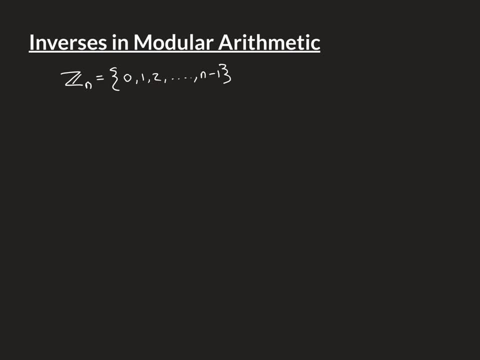 that congruence class will be represented by something back over here And that will be the answer to what your two elements added or multiplied together is equal to in our integers modulo n number system. So what we're interested in in this video is which elements inside the ring of integers 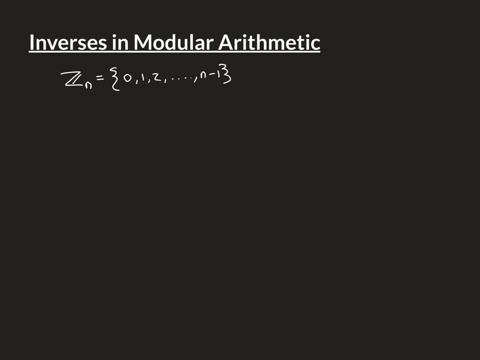 modulo n have multiplicative inverses. So if I take an element inside here, let's call it x. So x is an element inside z n, How do I know whether or not this element has a multiplicative inverse? So I'm going to give you the answer and then I'm going to explain why this is. 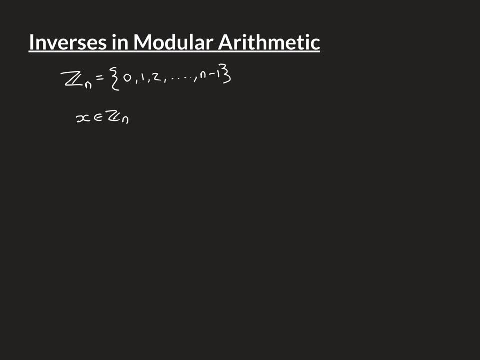 true. So x inside z n will have a multiplicative inverse inside z n if, and only if, it is co prime with the number n, where you're viewing both of them as integers. So of course n isn't an element inside your finite number system. So you have to step out of that. back to the 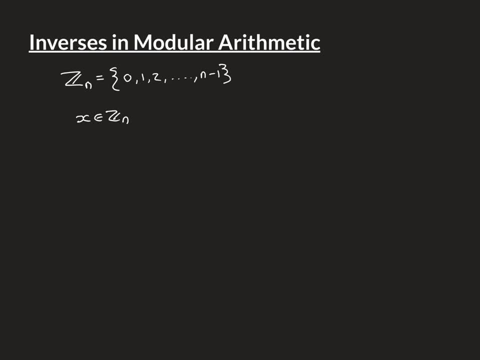 number system that we know and love, the integers. So what we're interested in in this video is the integers, And we know what greatest common divisor means in that context. So if the greatest common divisor of x and n is 1, ie they are co prime then and only then. 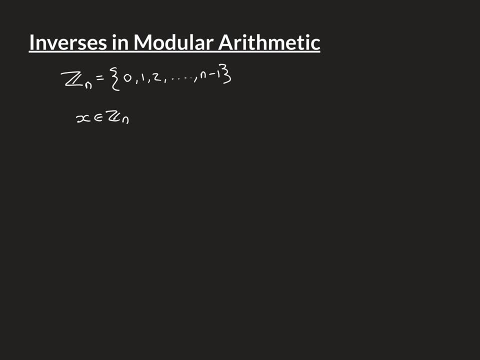 will x have a multiplicative inverse in the ring of integers modulo n. So we need the greatest common divisor of n and x to equal 1.. And a fancy bit of notation or fancy name for that is the two numbers n and x. n and x are co prime to one another, So I'm going to firstly prove that if this is the 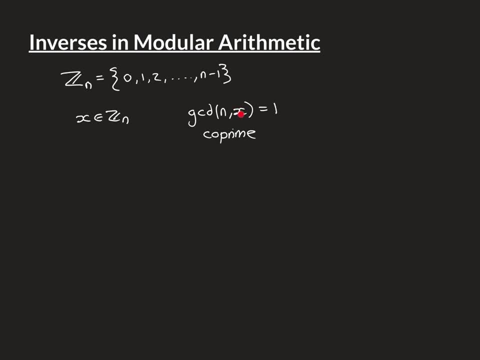 case, then x will definitely have a multiplicative inverse. And then what I'll show you is that if this isn't the case, ie if the greatest common divisor is some number bigger than 1, say 2 or above, then x won't have a multiplicative inverse in this ring. So this first bit is: 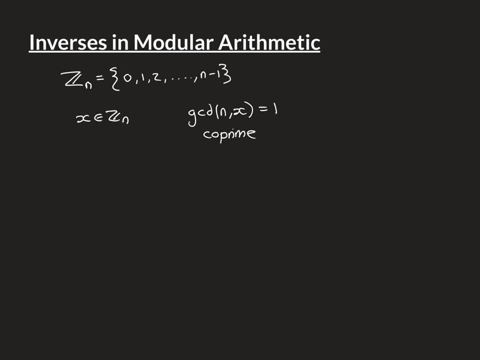 where we're going to use Bazut's identity. So, firstly, I'll just remind you what Bazut's identity says, but we're not going to prove it in this video. As I say, if you want the proof, go to the video on Bazut's identity. So Bazut's identity says that if you have, 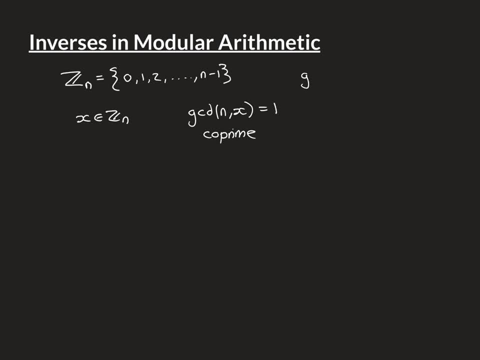 two integers, n and m, and the greatest common divisor of these two integers is equal to some value. let's call it d, then Bazut's identity gives you an equation that holds true in the ring of integers. It says that there are two integers that you can find. 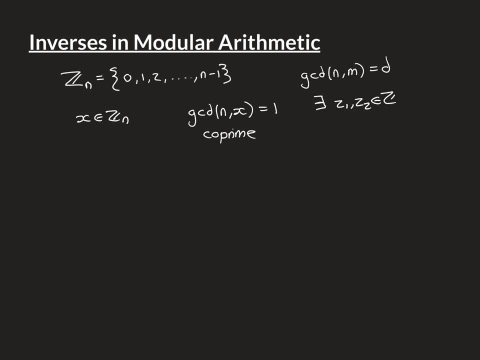 There exists z1 and z2.. z1 and z2 inside the integers, such that this equation holds true as an equation in the integers. So z1 times n plus z2 times m is equal to d. So what this is saying is: 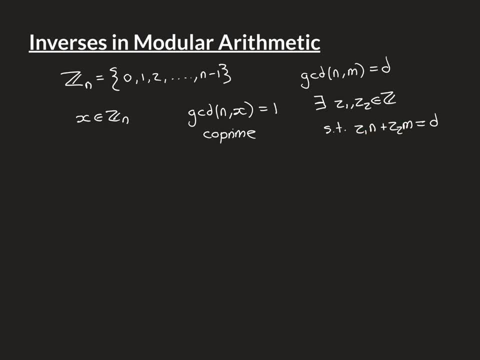 it's possible to find a multiple of n and a multiple of m such that if you add them together, the sum is the value of the greatest common divisor of n and m. Now we're going to apply this result here and indeed Bazut's identity, actually just. 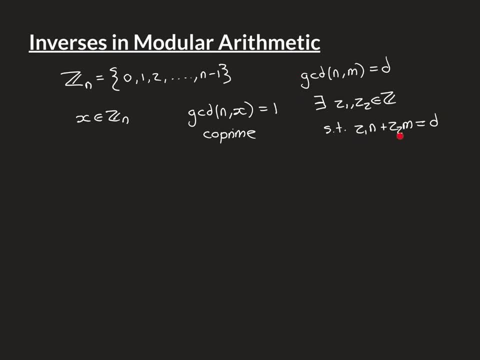 another little interesting fact gives you a way of actually finding these integers z1 and z2.. You can use the extended Euclidean algorithm to find these two. So we're going to apply Bazut's identity to what we've got here: the fact that the greatest common divisor 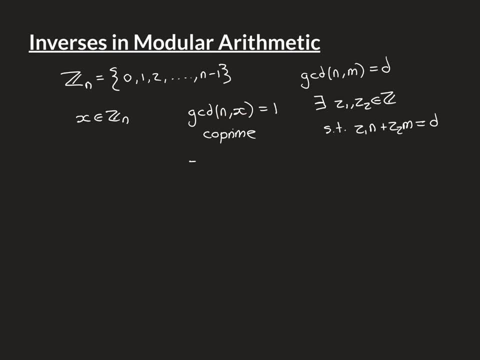 of n and x is equal to 1.. Now what we can consider is that, as an equation, in the integers there exists a z1 and a z2,, such that z1 times m plus z2 times x is equal to 1.. Now, how does this help us? Because 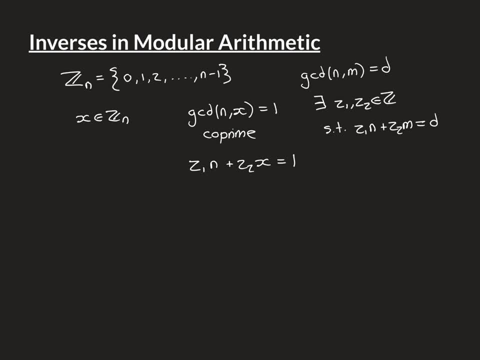 this is just an equation in the integers. We want to use this to infer something about what's happening in the integers modulo n. Well, what we can consider is: well, firstly, let's just rearrange this. We're very interested in this part because we've got something. 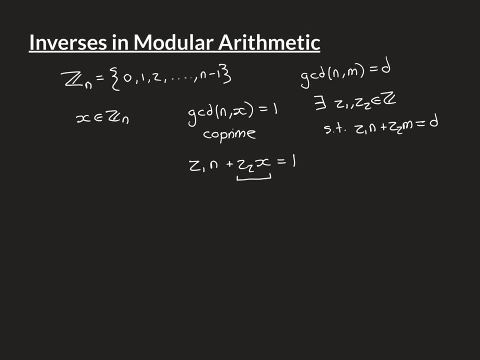 something times x, something in the integers. times x is equal to 1, and then if we move this bit to the other side, we'll have is equal to 1 minus z1 times n. So z2 times x is equal to this, But this is going to be something inside the congruence class of 1,. 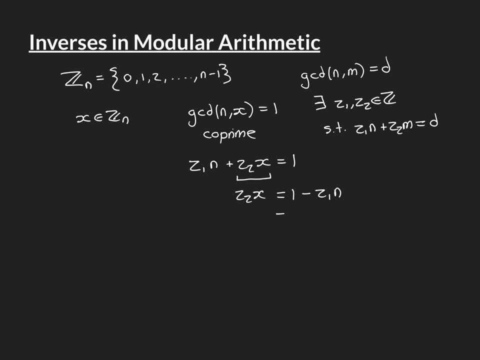 because it's 1 plus. and then let's swallow that minus 1 into the z1 here, So we'll have 1 plus, and then we've got minus z1 times n. So we've got minus z1 times n, So we've got. 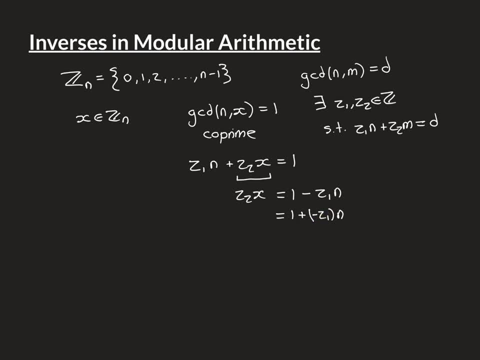 1 plus some integer times n. That is something that's going to be in the congruence class of 1.. Remember 1's congruence class, which we could denote 1 bar, or we could denote square brackets 1, or we could denote square brackets 1, and if we were being really formal, 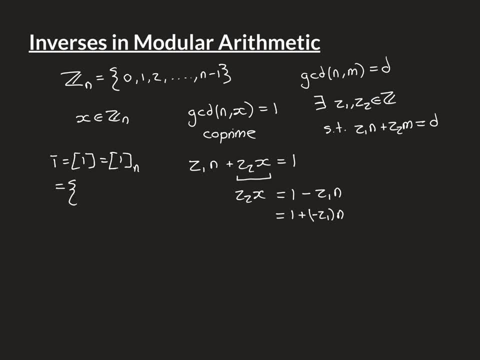 we'd subscript it. n is all the elements from the integers that are of this form: 1 plus z times n, Where z is allowed to vary over the entire integers. So you'd have 1 plus 0. lots of n. so you'd just have 1.. You'd have 1 plus 1, lot of n. 1 plus 2, lots of n. 1 plus 3 lots. 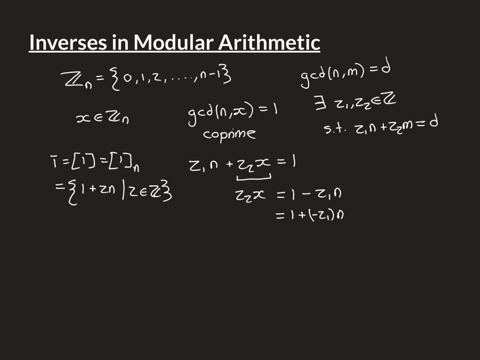 of n, 1 plus 4, lots of n. and then all the negatives as well: 1 minus n, 1 minus 2n, 1 minus 3n. all of them are going to be inside the congruence class of 1.. And this thing? 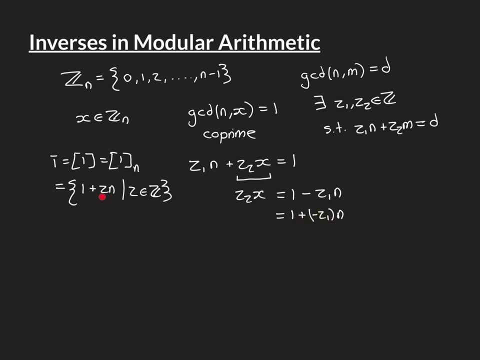 is going to be one of those elements, because minus z1 is some integer, so it's going to be something inside the congruence class of 1.. This is incredibly hopeful because you've got something. times x is giving you something that's inside the congruence class of 1.. So if this thing was inside here, then if we 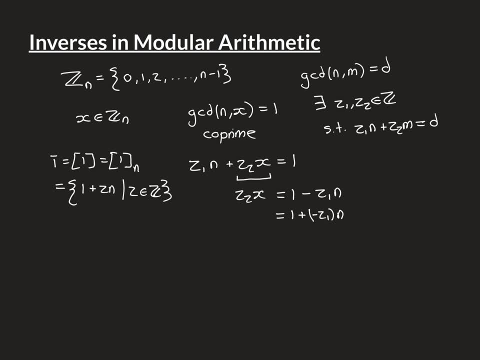 multiplied the two of them together. inside here it would be giving us 1 as the answer, because the answer in the integers is something that's inside the congruence class of 1.. Now the one little problem is that z2 might not necessarily be inside the congruence class. 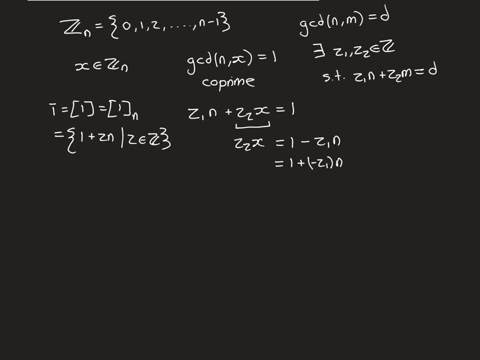 be inside here. However, we can get around that because Z2 is guaranteed to be in some congruence class of modulo m, So it's going to be in the congruence class of one of these elements, And when you multiply two things together using the congruence classes, we know that it's well. 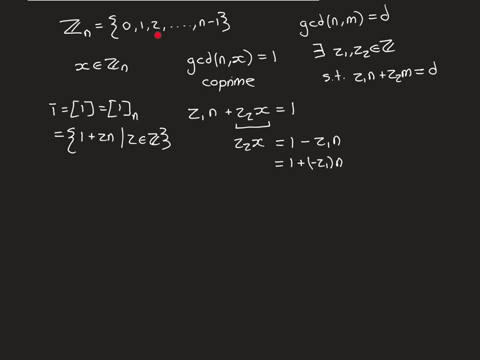 defined. so it doesn't matter what representative you pick. So if we can find something that's in the same congruence class as Z2 that is in here and we'll be able to do that, then that thing times x must give you something that's in this same congruence class as what Z2 times x gives. 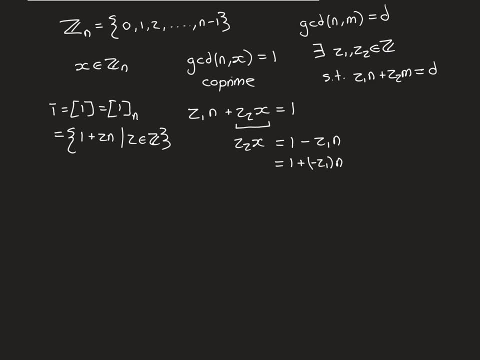 you, ie it will give you something that's in the congruence class of one. So let's go through this more slowly and write some of this down. So what we can say from this equation up here is that Z2 times x is giving. 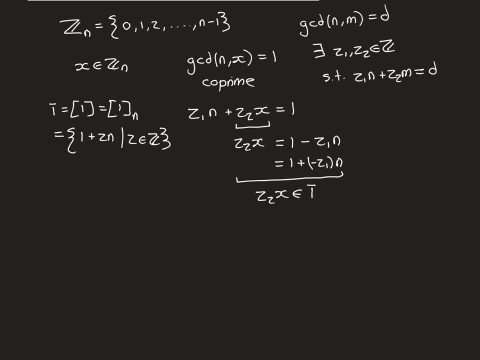 you something that's in the congruence class of one. It's giving you an element inside the congruence class of one. Now Z2, the big problem is that Z2 is just an integer. It's something in the integers, but it isn't necessarily one of these numbers that. 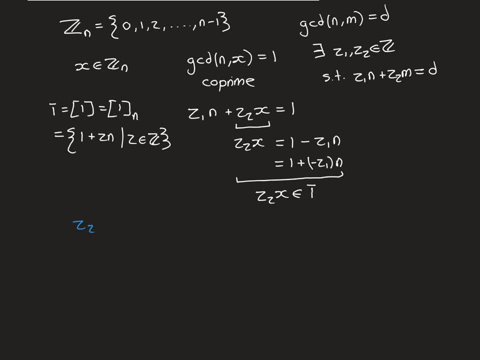 we've got in our integers modulo m. However, what we do know is that there must exist some element in here such that Z2 is in its congruence class. Let's call that element y. So there must exist a y- It's an element of Zn, such that Z2 is an element of the congruence class of y. And that's because the 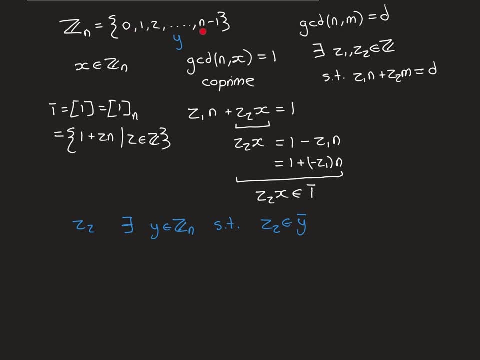 congruence classes. modulo n of all of these elements completely covers the entire integers. So just drawing a short picture to explain why that is the case: If we just draw the integer number line like so, So here's zero, that say and here: 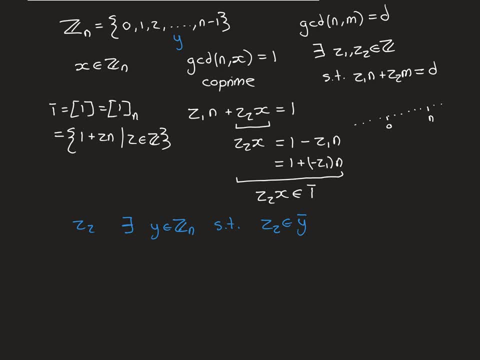 is n, then the congruence class of zero is all multiples of n, integer multiples of n. So you'd have n, 2n, negative n over here and onwards You'd have negative two, n, three, n, et cetera. 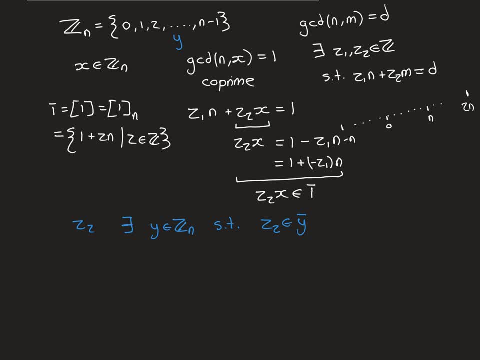 and then, if we look at the congruence class of one, it's all things of the form one plus zn, so it's gonna have one plus n, one plus nn plus 2n, 1 minus n, etc. If we look at the congruence class of 2 in blue, it's all the. 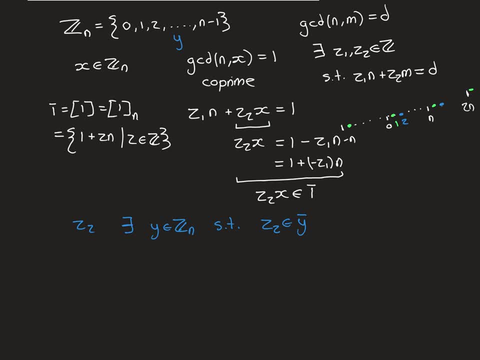 things of the form 2 plus Zn, So you'd have 2, 2 plus n, which is here, Then you'd have 2 plus 2n. 2 minus n will be over here And you can see that as you continue on from 0. 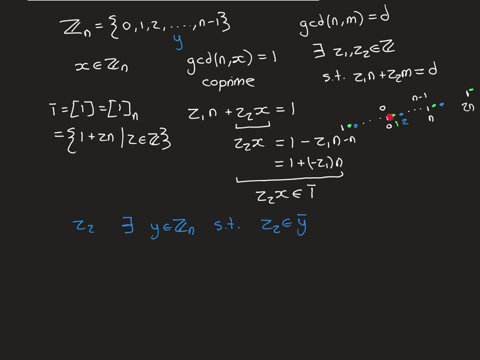 here to n minus 1 here. if you go through all of their congruence classes, it's going to fill in all of these gaps so that the whole of the integers is covered. So wherever Z2 is- and it might be, you know completely off this picture. maybe it's over here. it. 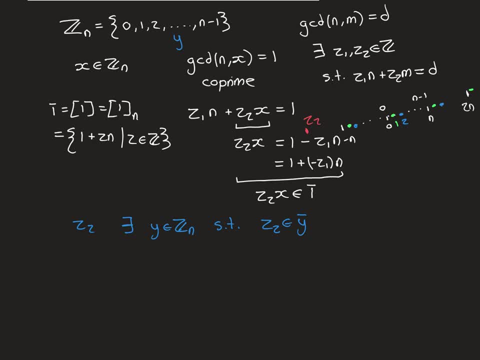 will be inside one of these congruence classes. So there will exist some y, maybe this one here, such that when you look at its congruence class, it contains Z2.. So that's what we're saying here. There is 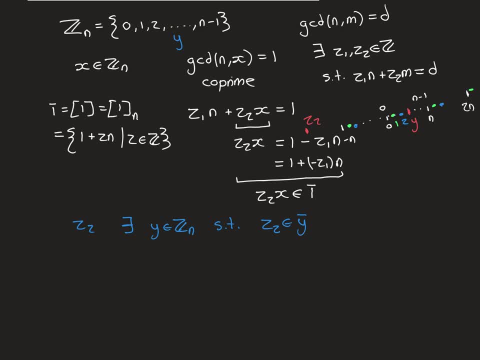 There is some element inside here, such that Z2 is within its congruence class. Now I claim that y is now the element inside the integers modulo n, that is the inverse, the multiplicative inverse, to x. The reason being is that if you multiply y and x together the way you, 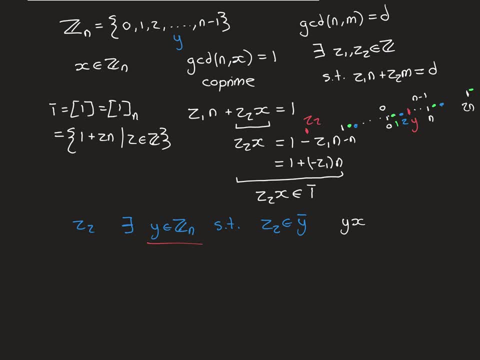 do this is by going to their congruence classes. So you look at the congruence class of y and the congruence class of x and you take representatives. You take the representatives from those and you could take the representative Z2 from. 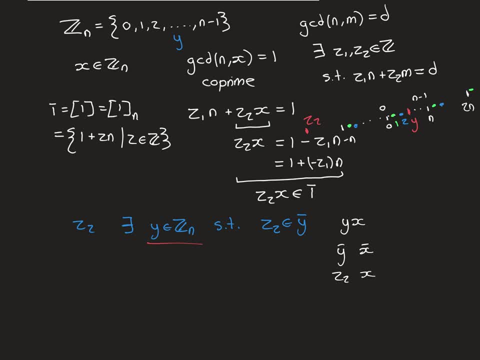 the congruence class of y and you could take the representative x from the congruence class of x. You multiply these two together in the integers and then you look at what congruence class is the answer in, and we've already said that the answer to that is in the congruence. 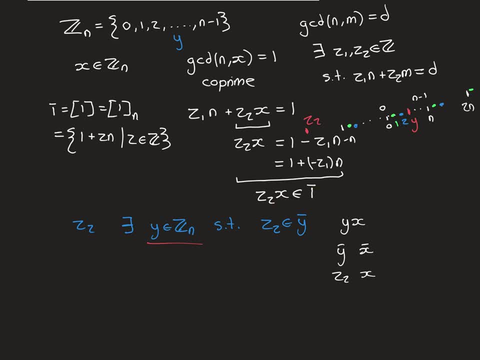 class of one, And then you take that things, the thing in here whose congruence class you're in, as the answer. So you're in, therefore one's congruence class, and therefore y to x is equal to one, which means therefore that y is the multiplicative inverse of x. 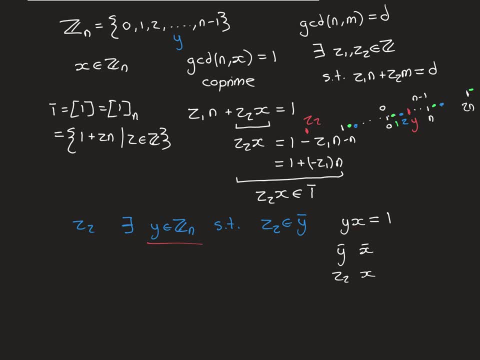 because that's the definition of the multiplicative inverse of x, that you multiply together to give one. Both ways of course needs to be true, but that clearly is going to be true. if we do it the other way around- x times y- Then we can use the exact same argument. 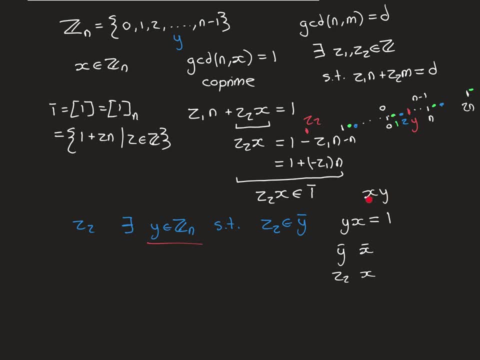 Pick Z2 as your representative of the congruence class of y. Pick x as your representative of the congruence class of x. Multiply them together in the integers, and we know the integers are commutative, so you're still going to get the same answer, ie an element of the congruence class of one. 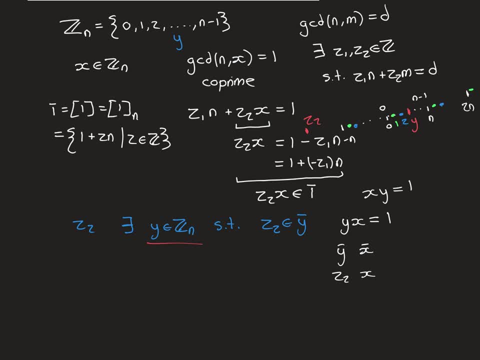 So xy is also going to be equal one. So we therefore know that y multiplied with x in our integers, modulo n is going to give one both ways around, and therefore y is the multiplicative inverse of x. So that completes our proof, then, that if x and n are co-primed to one, 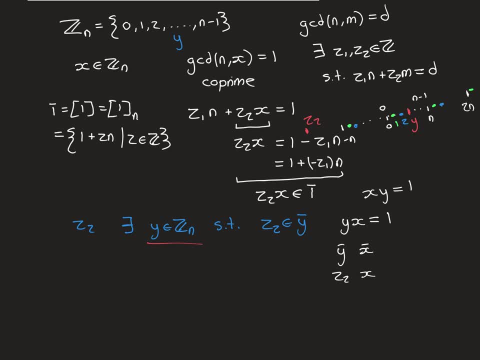 another, then x will have a multiplicative inverse inside the ring of integers modulo n. And just before we move on, let me emphasise that the incredible thing about the ring of integers modulo n that makes all of this possible is the fact that addition and multiplication. 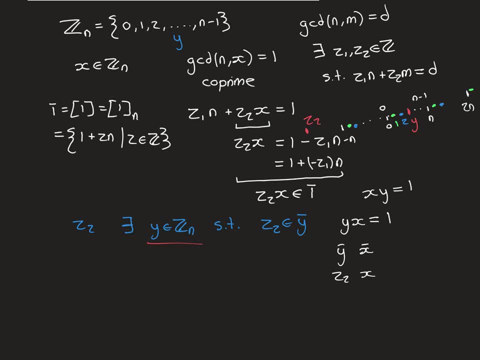 are well defined. So whatever two representatives you pick from the two congruence classes. so if we're, for instance, multiplying y and x, whatever representative you pick from the congruence class and whatever representative you pick from the x congruence class. when, 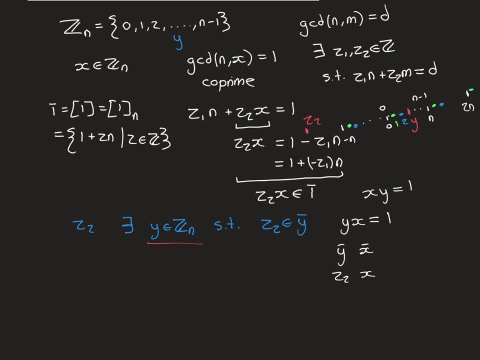 you multiply the two representatives together in the integers, you'll get a different answer depending on which representatives you pick. However, the answer will always be in the same congruence class, so the answer of what the overall congruence class you're in remains. 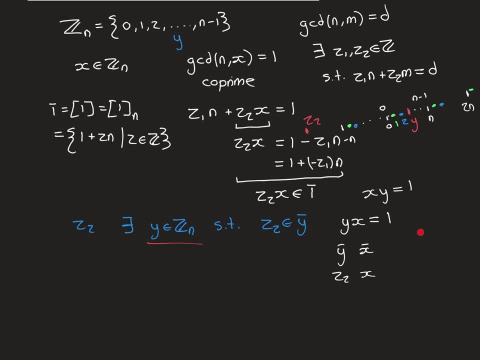 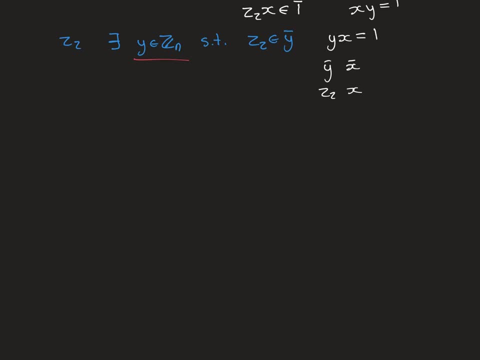 the same. It is well defined. So that's obviously crucial to what we did here. So let's move on now. So let's move on now. Let's now look at the case where the greatest common divisor of x and n is not 1, so it's. 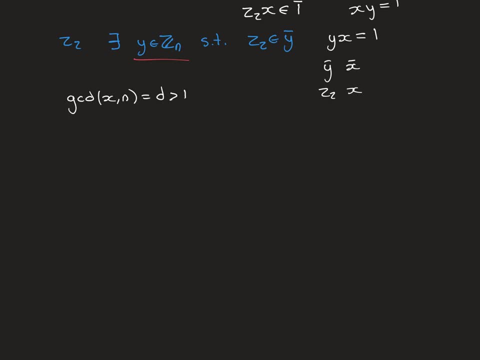 instead equal to some d, where d is strictly greater than 1.. It is of course still an integer, And we want to see how. in this case it cannot be possible for x to have a multiplicative inverse modulo n. So the way I'm going to disprove this is by contradiction. So we'll 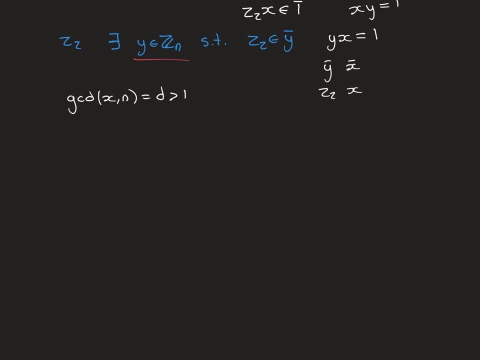 suppose, for the sake of contradiction, that it does have a multiplicative inverse modulo x. So we think x root x must be vector bias of the integration v of x. So x is the derivative which of 2 is derivative of 2.. So instead, what happens is that the next step in multiplying as duplicative 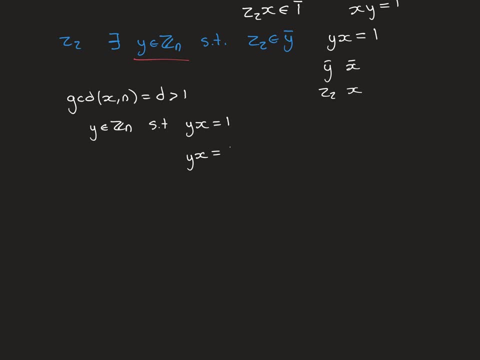 inverse turns out to be a similar equation, and it is in this case y- controlled. You can see that y- is equal to 1 in the congruent class of x. So you will首み all thechez though n. That means it must be equal to 1 plus z times n, where z is some integer, That's. 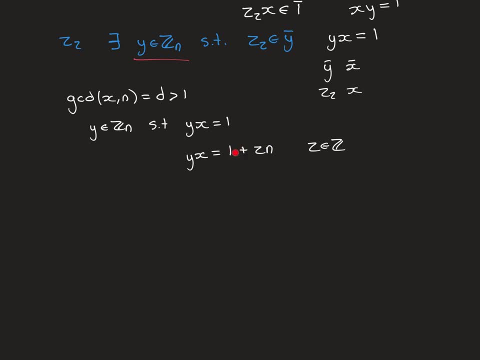 what it means for y times x in the integers to be in the congruence class of 1.. These are all the elements inside that congruence class of 1, so it must be equal to one of them, so it must be equal to something. There must be a z that makes this true. Now this: 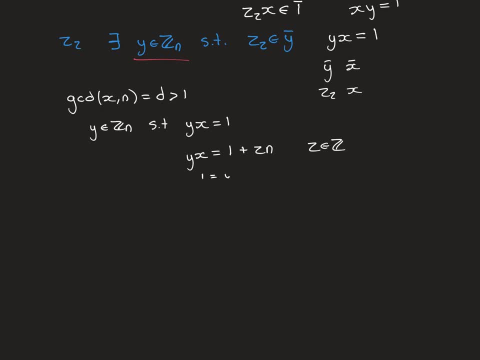 is a problem because we can rewrite this as: 1 is equal to y times x minus z n. That's a perfectly valid manipulation inside the integers, And what we know is that the greatest common divisor of x and n is equal to this value, d that is greater than 1.. So we know. 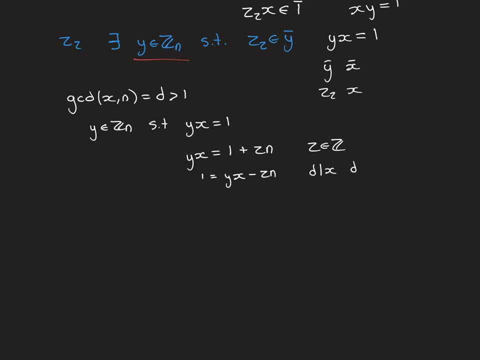 that d is a common divisor of x and n, so d divides x and d divides n. That means that x can be written as some multiple of d, some integer multiple of d. we'll call it n1 times d, and n can be written as some integer multiple of d. 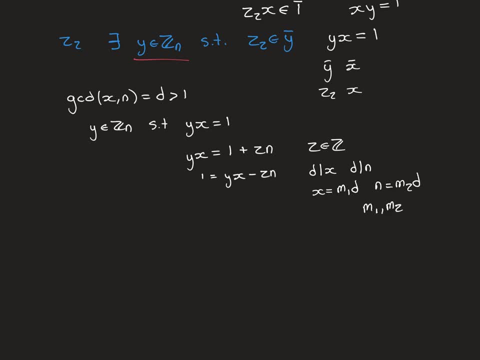 Now we'll just put those into this equation and we're going to get some garbage. So 1 is equal to y, whatever, that is the thing that can't exist. times n1 times d minus z. times n2 times d. Now I'll just pull out that d and we get this is y times n1 minus z times. 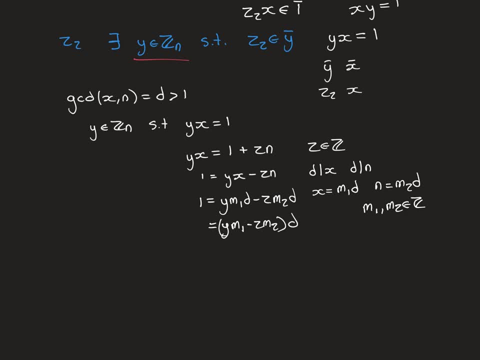 n2 times d. Now this is an equation in the integers. y is an integer. Remember it was just some number inside z, n, so it was an integer. It was some number: 0,, 1,, 2,, all the. 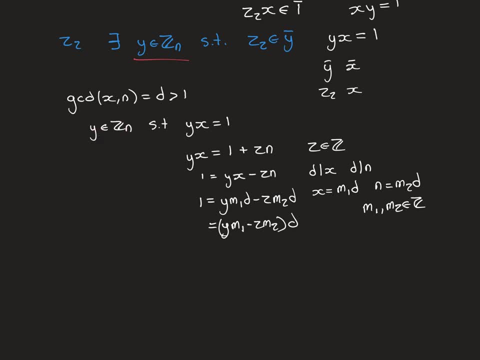 way up to n minus 1.. It was one of those, but it transferred across into the ring of integers. So then we multiplied it by another integer, then we subtracted off two other integers multiplied together. This is all algebraic operations inside the integers. 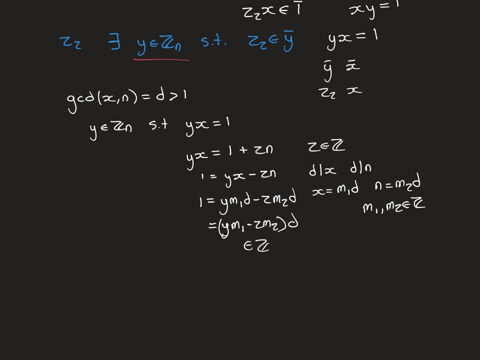 so it's going to come out as some integer. So this is then saying that some integer times some number that is greater than 1, so some positive integer bigger than 1 is equal to 1.. Well, that's nonsense, We know. 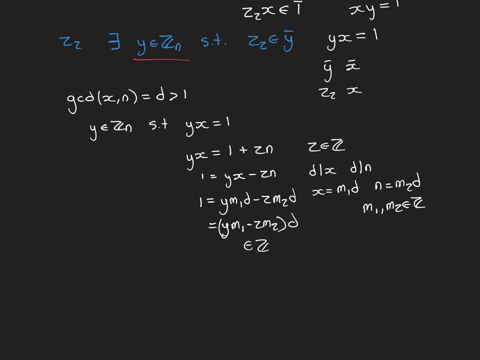 inside the ring of integers, there are only two elements with multiplicative inverses: 1 and negative 1.. All of those positive integers bigger than 1 do not have multiplicative inverses. If this was true, this thing would be the multiplicative inverse of d. Imagine d is. 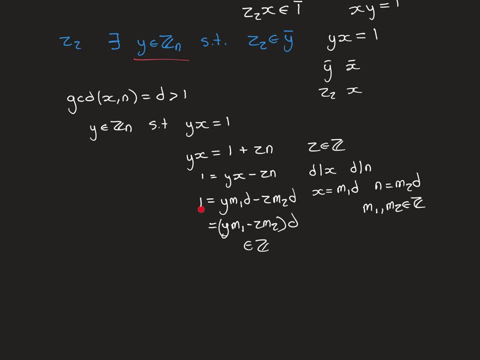 3. There is no integer that multiplies by 3 to give 1.. You know, because if you multiply it by 0, you get 0. If you multiply it by any negative integer, you're going to go into the negatives. You're not going to be equal to 1.. If you 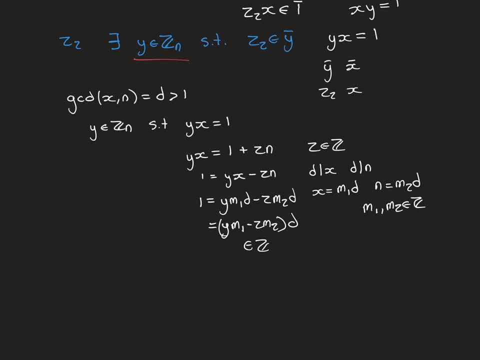 multiply it by 1, you get d. If you multiply it by 2, you get 2d. You know these are all getting bigger and bigger. They're never going to come down somehow magically to 1.. So this is nonsense. This can't be correct, And therefore we go back to our initial assumption that 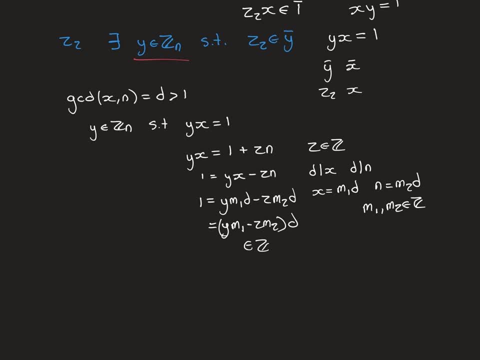 there was some multiplicative inverse for x and it must have been wrong. So therefore it's proven that if the greatest common divisor of x and n is greater than 1, ie they're not coprime to one another- then x cannot possibly have a multiplicative inverse in. 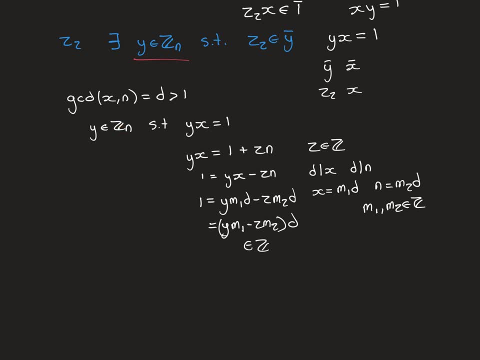 the ring of integers modulo n. So it is the case that if they are coprime, then x will have a multiplicative inverse, and if they're not coprime then it won't have a multiplicative inverse. So it will have a multiplicative inverse if, and only if, x and n are coprime. 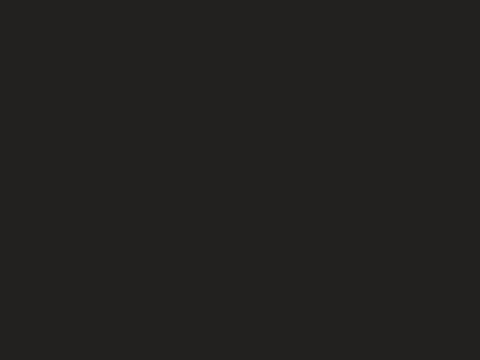 to one another. Now, before we end, I want to thank you for watching this video. I hope you enjoyed it and I'll see you in the next one. Bye for now. So we'd just like to do an example of applying this to an actual, concrete example. So I'm 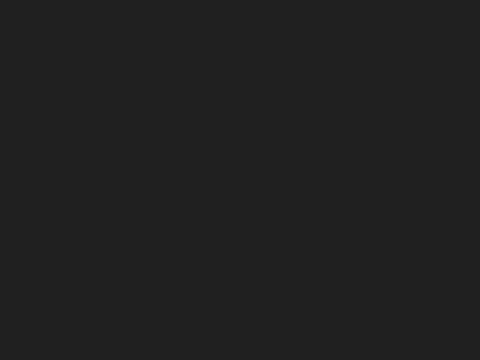 just going to come up with some numbers. So we'll take 9 and 14.. So we'll take the ring of integers modulo 14, and then I'm going to look at the number 9 inside there. So of course, this is a set is 0,, 1,, 2,, all the way up to 13, with its addition and multiplication. 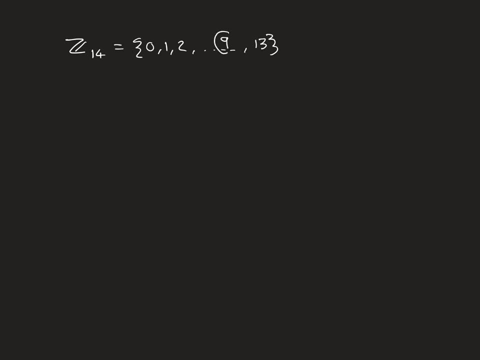 and composition laws on it. I'm going to be interested in this number, 9, and I'm going to do more than just find the multiplicative inverse of 9.. I'm going to actually solve an equation inside this number system. So let's say we have the equation: 9 times x is. 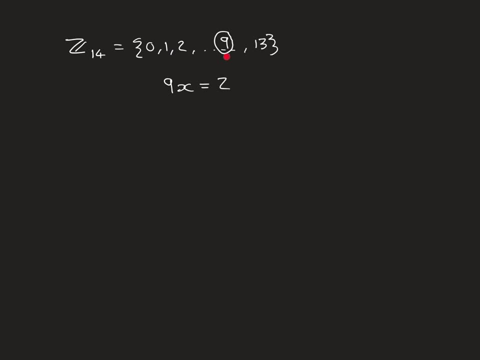 equal to 2.. That's a perfectly valid equation inside this number system: 9 times some value. so I'm asking: can you find, are there any solutions to this? Is there any x inside this number system Satisfies this, such that 9 times that x is equal to 2.. Well, if 9 has a multiplicative 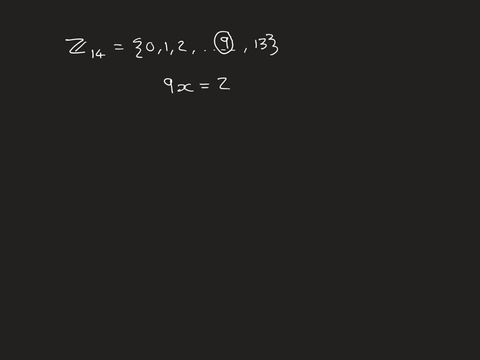 inverse inside. here we could solve this just by multiplying both sides by that multiplicative inverse. Then, by the associativity of multiplication, we could multiply 9 with its multiplicative inverse to give 1, and then we get x is just equal to the multiplicative inverse of 9 times. 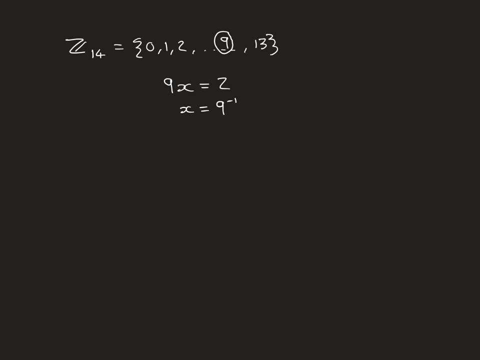 2.. So this is going to be the multiplicative inverse of 9,, if it exists, times 2.. And what I'm going to show you is that it does exist In this case, and I'm even going to find its multiplicative inverse using the extended 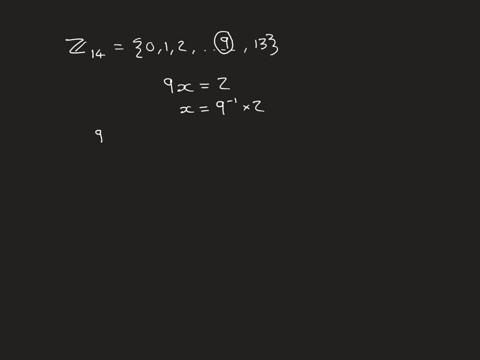 Euclidean algorithm. So 9 and 14,. the greatest common divisor of 9 and 14 is indeed 1.. So they are going to be co-prime. You can write 9 as its prime factorization, which is 3 times. 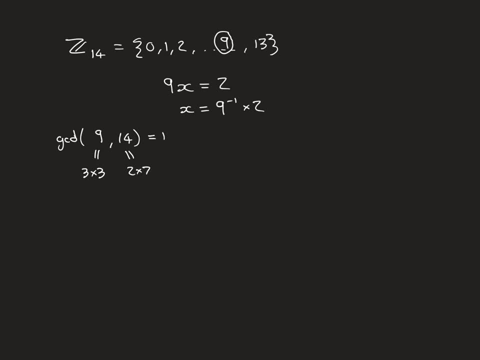 3, and 14 as its prime factorization, which is 2 times 7.. So they are going to have no common factors. So what we're going to do is apply the extended Euclidean algorithm to find the coefficients in Bazut's identity for 9 and 14,, and that will yield us the multiplicative inverse of. 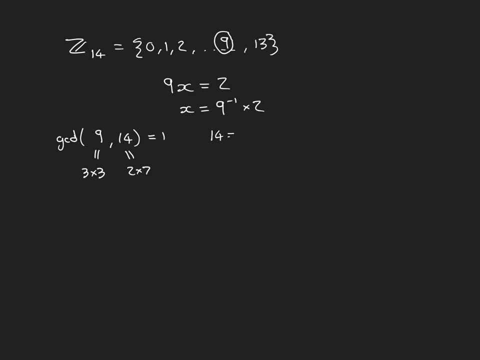 9.. So, doing this, 14 is equal to 1 times 9 plus 5, is the first line of the Euclidean algorithm. Rewriting this, we'll have that 5 is equal to 1 times 14 minus 1 times 9.. 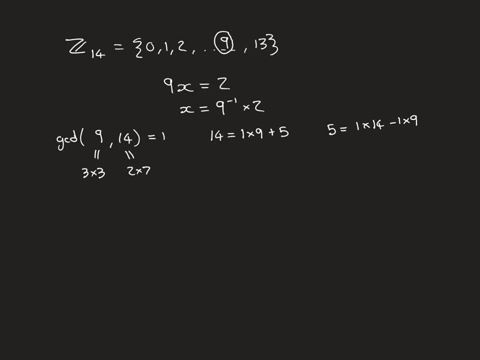 So I'm assuming that you're familiar with how to perform the extended Euclidean algorithm. If you're not, it's in previous videos in the playlist on number theory, Next 9, we'll have that 9 is equal to 1 times 5 plus 4.. We'll rewrite this: 4 is equal to. 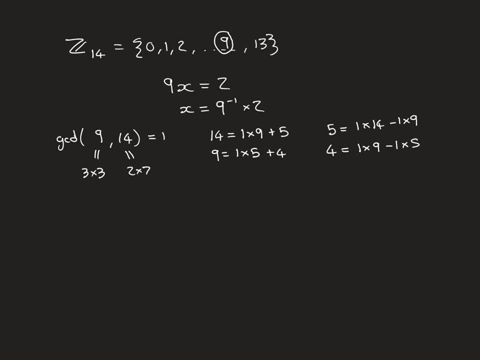 1 times 9 minus 1 times 5.. And then we don't like this because we want equations completely in terms of 14 and 9.. At the moment, we've got an equation in terms of 14 and 9.. We don't want this. We want an. 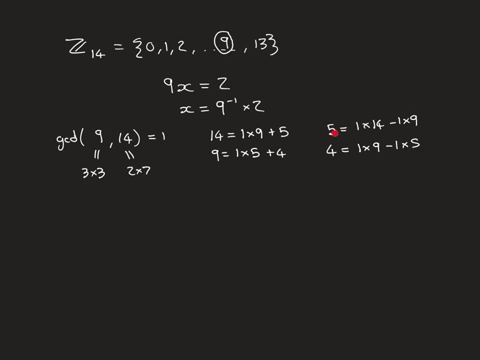 equation that is completely in terms of 14 and 9.. We want an equation that is completely in terms of 14 and 9.. We want an equation that is completely in terms of 14 and 9.. Because we're 9 and 5, but that's okay. We can substitute this equation that we've got for 5 into here. 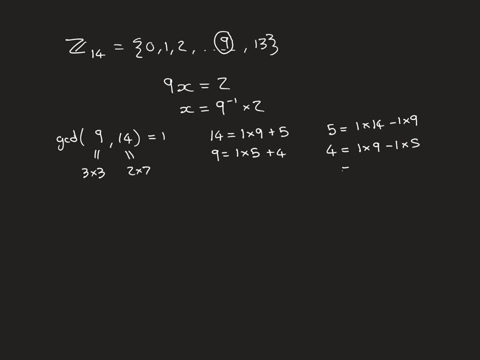 and we'll then have an equation in terms of just 9s and 14s. So this is going to give. we'll have 1 times 9, and then minus 1 times minus 1 times 9.. So that's going to give. 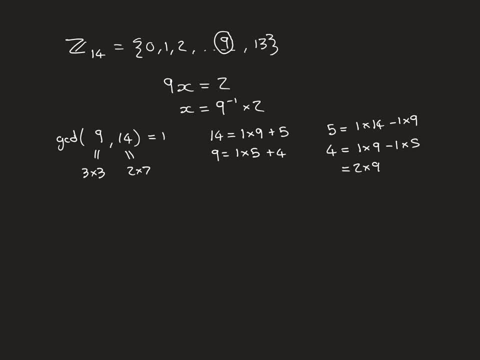 another 1.. So we'll have 2 times 9, and then minus 1 times 14 overall. And let's just do a check of our calculation here: 2 times 9 is 18, minus 1 times 14 is indeed 4.. Good. 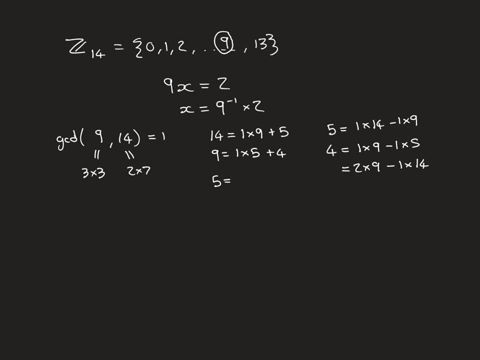 Let's continue on. Third line of the Euclidean algorithm is going to be: 5 is equal to 1 times 4 plus 1.. And then the final line will just be: 4 is equal to 4 times 1.. So indeed, 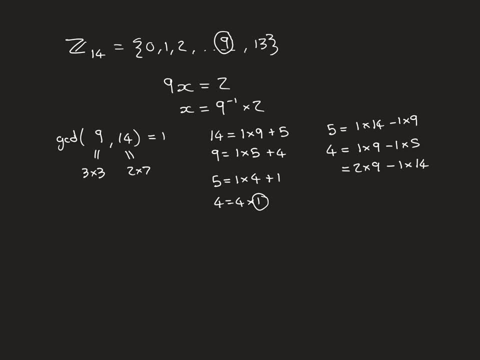 1 is the greatest common divisor by the Euclidean algorithm. here Let's do the next line of the extended Euclidean algorithm. It will give: 1 is equal to 5 minus 1 times 4.. So now just substitute both of these equations that we've got for 5 and 4 in terms of 9 and 14,. 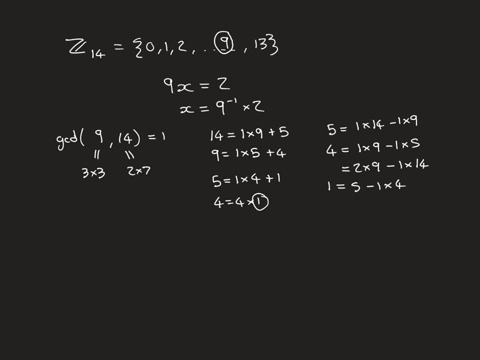 and we'll get 1 times 4 minus 1 times 4.. So now just substitute both of these equations that we've got for 5 and 4 and we'll get an equation for 1 in terms of 9 and 14.. So this gives us: 1 is equal. 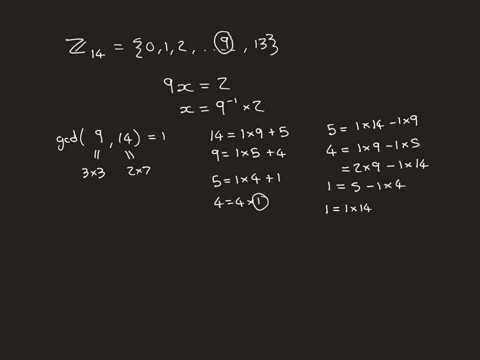 to so. substituting in 5's equation, we've got 1 times 14 minus 1 times 9.. Putting in 4's equation, we'll get minus 1 times 2 times 9.. So that'll give plus minus 2, minus 2 times 9.. And then we'll have. 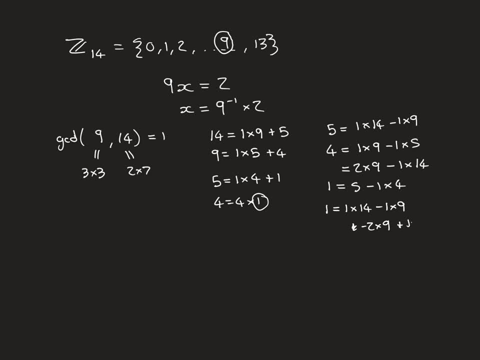 minus 1 times minus 1 times 14, which will be plus 1 times 14.. So this overall comes out as 2 times 14 minus 3 times 9.. And let's just check that: 2 times 14 is 28.. 3 times 9 is 27.. So 28. 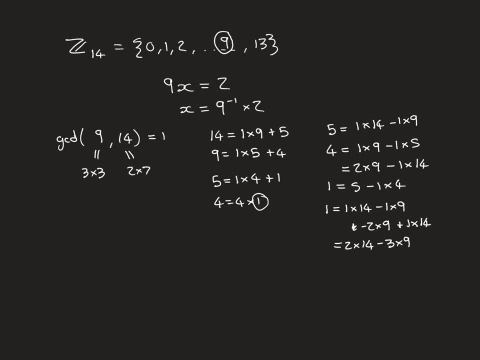 minus 27 is indeed equal to 1.. So now this, this is Bazut's identity. These are the coefficients. So one of the coefficients is 2 in front of 14, and one of the coefficients is minus 3 in front of 9.. 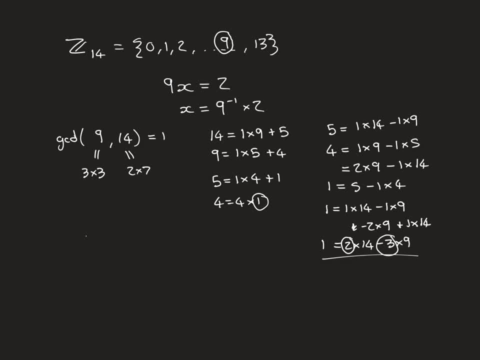 And we can now use this to find 9's multiplicative inverse, because, looking at this, we've got minus 3 times 9, is equal to 1 minus 2 times 14.. So it's saying, if we multiply negative 3, 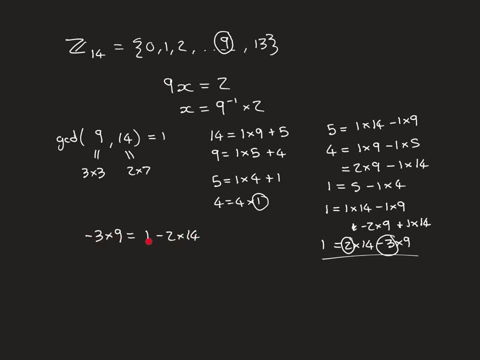 by 9, we get something inside the congruence class of 1 modulo 14.. And this is a problem because minus 3 isn't exactly in our integers modulo 14.. So we just need to find what congruence class is. 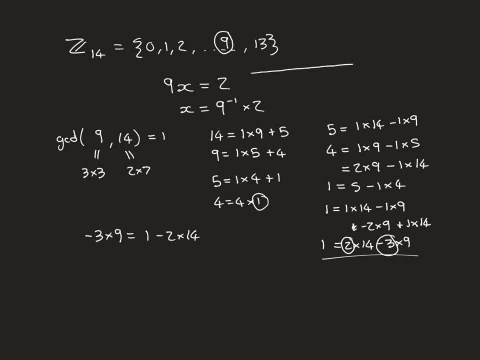 it in. So, thinking about the number line, so you've got 0 here and I have drawn the continuous number line which usually represents the reals. but we'll just think about the integers. here We've got 14 here. We've got minus 14 here. 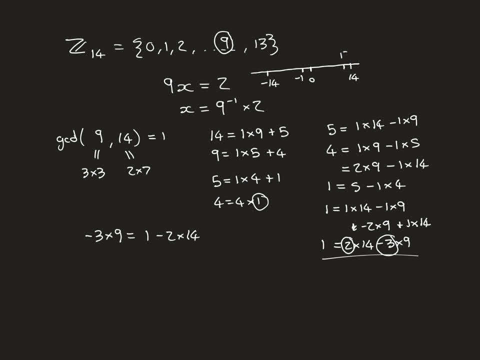 When you go backwards to minus 1, that is in the same congruence class as 13.. When you go to minus 2, that's in the same congruence class as 12.. When you go to minus 3,: 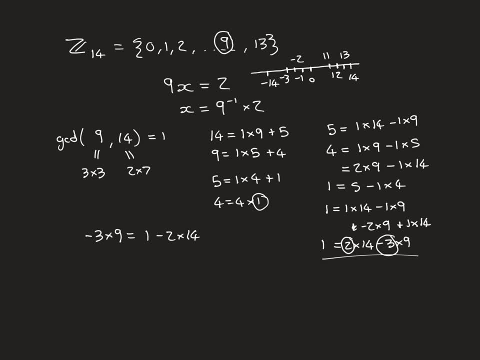 that's in the same congruence class as 11.. So minus 3 is in the same congruence class as 11, so that means that if we multiply 11 by 9 inside here it will give us 1.. So 9 times 11.. 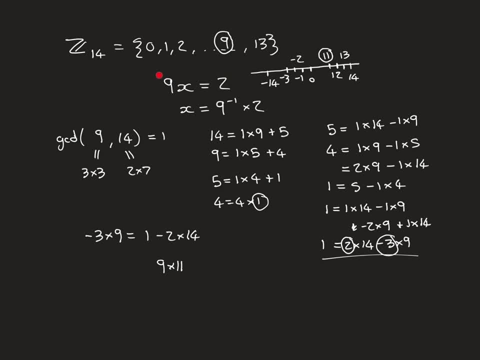 Oh, and, by the way, something that I will just tell you, I've been writing this in this way. Notation that you will see people use when they are doing modular arithmetic is the old notation, but it's still commonly used. You will often see people writing this instead with the: 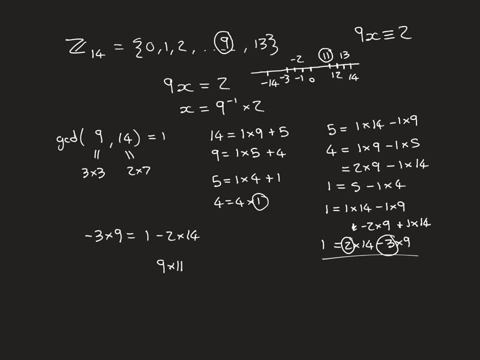 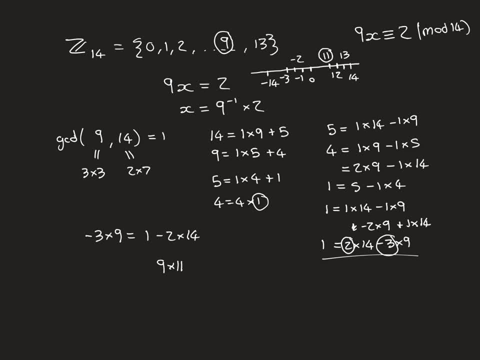 even write in brackets more to the 14.. This notation is very common. I don't like it as notation because it implies that this is a less good number system. It implies that it's not a number system. in a way, It implies we're just talking about the integers with 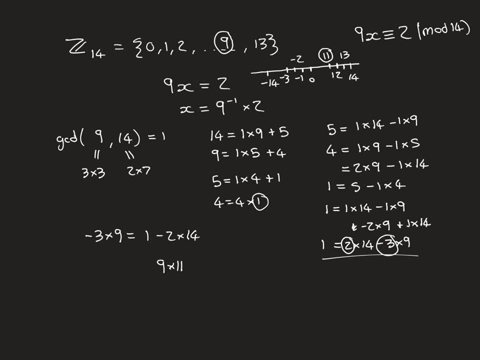 talking about congruences instead of actually giving this, treating this with respect as a number system in its own right. So I actually prefer to just write this and say: we're working now in this finite number system and we want to solve this equation. But you often will see things like this written: 9x is congruence to 2, modulo 14,. 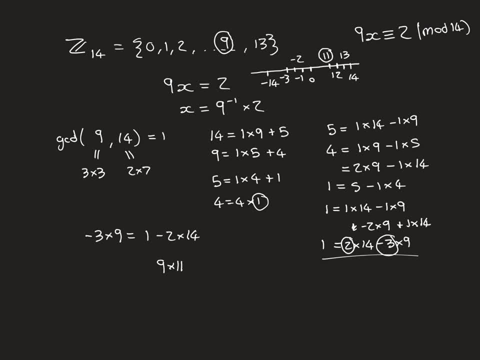 and you'll be asked to solve this congruence equation. But it is effectively just a number system in its own right and we're solving an algebraic equation in this number system. But this notation was invented years before the advent of abstracts. 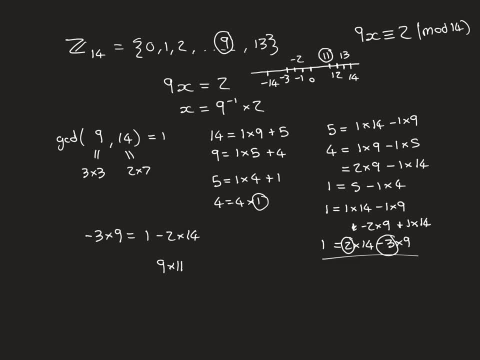 abstract algebra and it is still in use And you'll more commonly see that written even than this. Anyway, where were we So 9x11,? I was prompted to think about that because I was going to put in brackets here modulo 14, so we're doing 9x11 in our 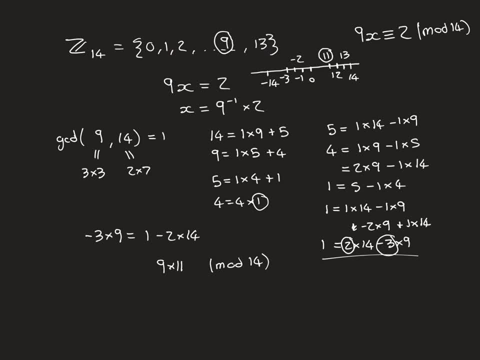 modular number system here. So the way that you could do that is, you would take representatives from these two congruence classes. We could take 9 and 11, multiply them together in the integers and we'd get 99. And then 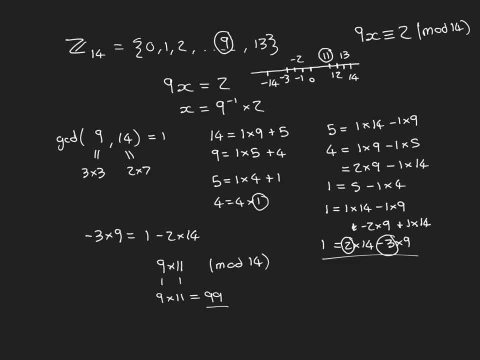 we just need to figure out what congruence class that is in. But we know we're guaranteed to get this right. because another thing: in the congruence class of 9 is negative 3.. Sorry, not in the congruence class of 9.. In the congruence class of 11 is negative 3.. And we know that. 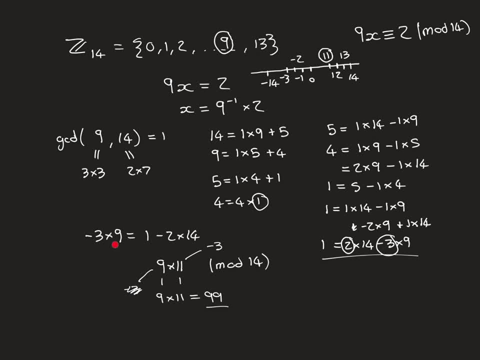 if we multiply 9 with negative 3 in the integers, it gives us this thing: 1 minus 2 times 14, which is in the congruence class of 1.. So because we know everything works and is well-defined, 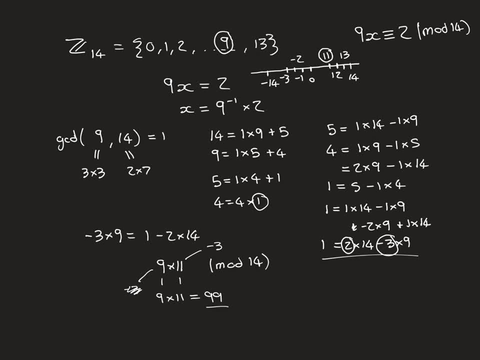 we know we're guaranteed to get in that congruence class, But let's just check this. So 99, we just now need to multiply 14 by something. So let's try 14 times 5. firstly, This will give us 70. So let's do 14 times 6.. That will give us 84.. 14 times 7 will give us the. 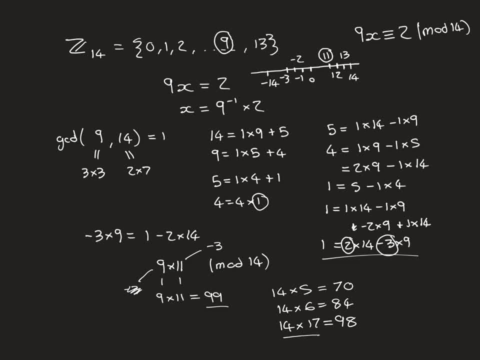 bang-on number 90.. So 14 times 7 is equal to 98.. So adding 1 onto that, you get 99. So this is actually equal to 1 plus 7 times 14. So indeed, 9 times 11 gives us something that is in the congruence. 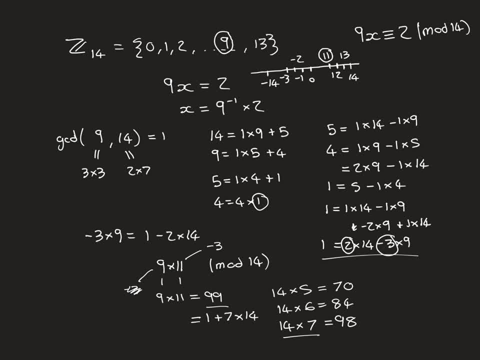 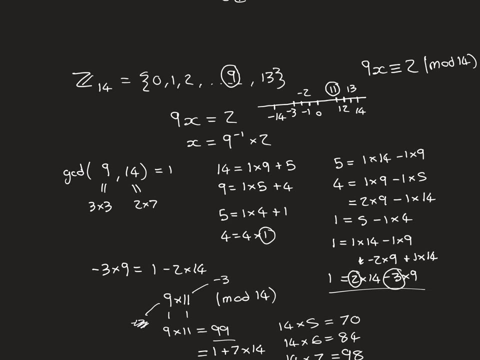 class of 1, modulo 14.. So, yes, this is all working As we knew it must do, because with this other representative of that same congruence class, it was giving something inside 1's congruence class. So what we can now do, going back to our original, 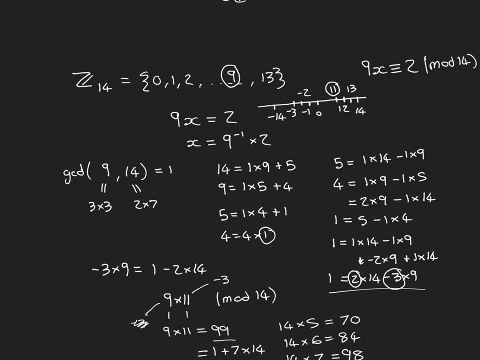 equation. if we want to solve this equation, we now know what 9's multiplicative inverse is inside here It's 11.. So we can now multiply both sides by 11.. This side, multiplying by 11, will give 1. So it goes. So we then get that x is equal to 11 times 2. So we now know. 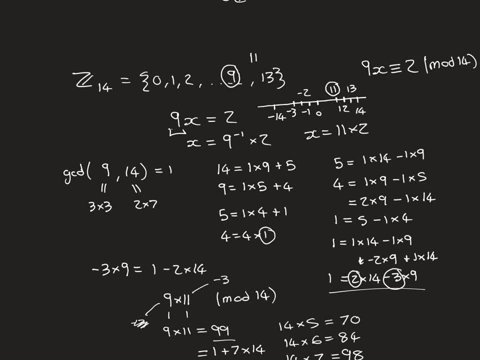 that x is equal to 9 times 2.. If we want to work out what that is, again, we take representatives from the congruence classes. So we'll just take 11 and 2, multiply them together in the integers, we get 22.. And then we just need to ask: what congruence class is that in? Well, 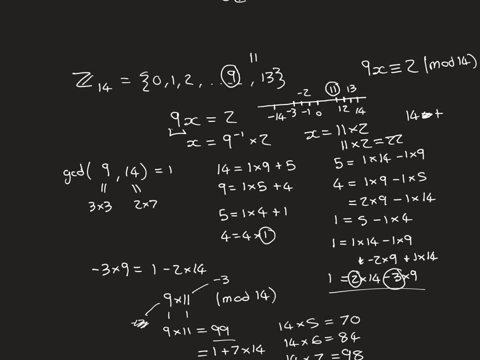 22 is equal to 14 plus 8.. So it's therefore going to be in the same congruence class as 8.. So the answer is: x is equal to 8.. So if you take 9 and multiply it with 8 inside here, 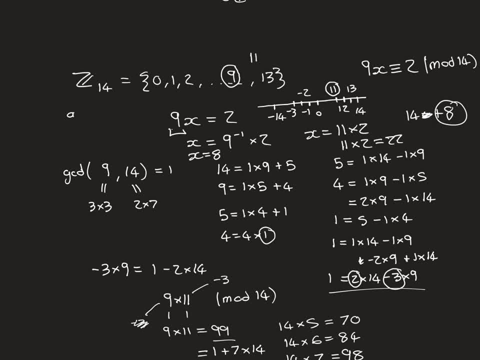 you'll end up with 2.. So you can see that x is equal to 9 times 8.. So you can see that again, it's going to be in the congruence class of 2.. We can finally just check that So. 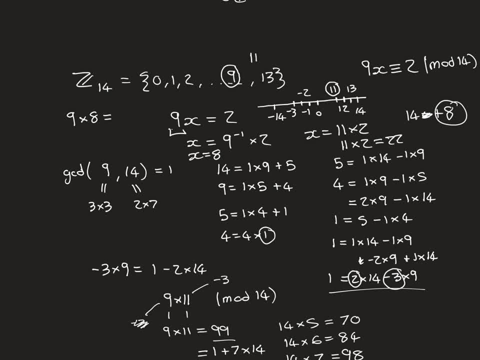 9 times 8, take the representatives in the integers 9 and 8, multiply them together. Gosh maths. What is 9 times 8?? 9 times 9 is 81. So 9 times 8 is 72. And then we can. 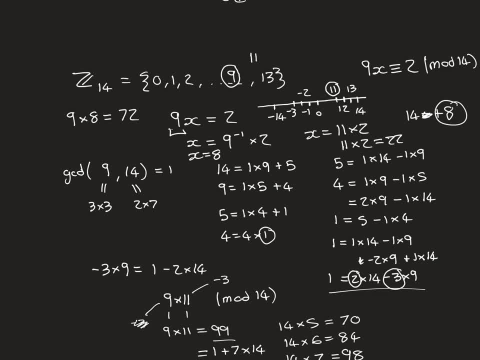 use what we've got down here. We know that 14 times 5 is 70.. So this is 14 times 5 plus 2. And therefore it's in the congruence class of 2.. So the answer is 2.. 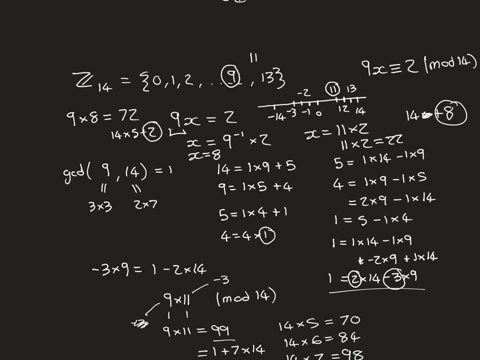 answer is 2 modulo 14.. So it works all beautifully. So if an element is co-prime to the n that the integers is modulo, then it will have a multiplicative inverse. If it is not, then it will not have a multiplicative inverse. And this is how you can find multiplicative. 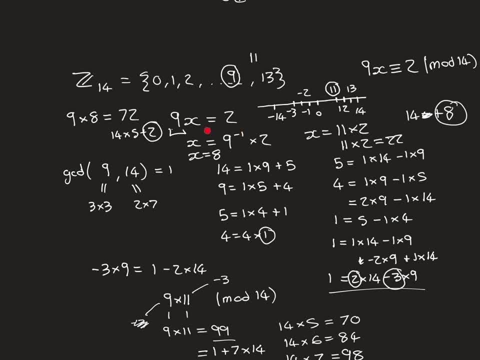 inverses using the extended Euclidean algorithm and how you can use them to solve these sorts of equations in modular number systems, sometimes called congruence equations.